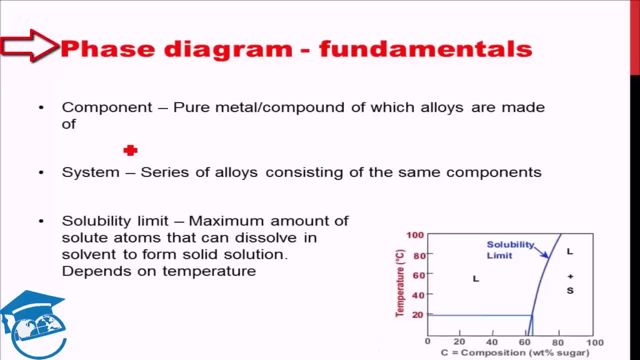 So one of the things that you will encounter many a times when discussing about phase diagrams and phases is known as Component, OK, Component, Okay, OK refers to a pure metal or compound out of which alloys are made. okay, So it is either a pure metal or a compound. 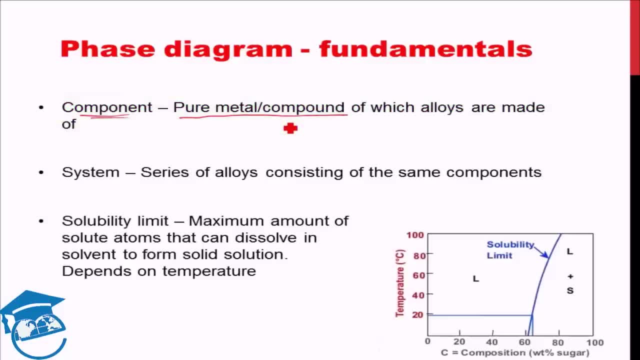 Now, in order to give you idea about each of these terms, I will be using a simple example of sugar water solution. okay, A sugar water solution. Using this, we will understand each of the terms which we will define here. So, in a sugar water solution, the components are sugar and water. 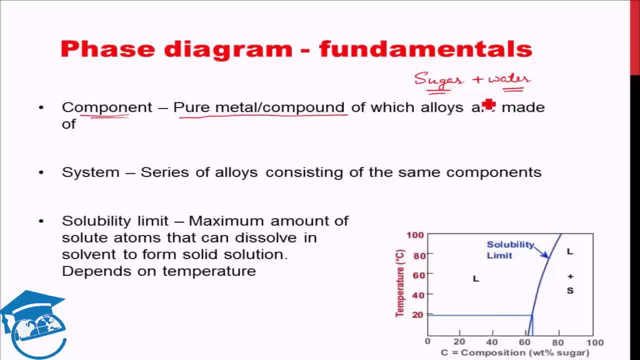 These are the two components present in a sugar water solution. fine, Now system. What is a system? System can be referred to as a series of alloys consisting of same components. What do I mean by this? What I mean is that, again using the sugar water example, you can have 10% sugar in water. 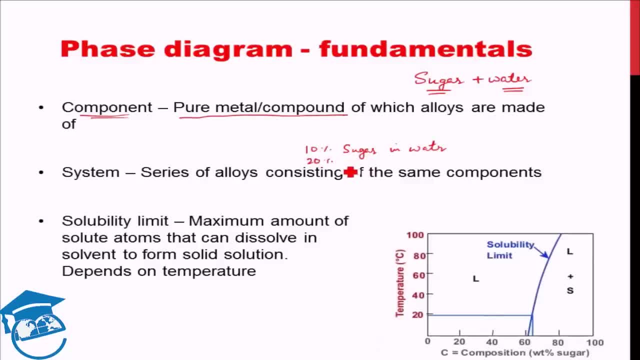 or you can have 20% or 30 or 25.. So there are different combinations of sugar and water amount that can be present, right? So this is a series of alloys we normally use in metals, but here we can say series of mixtures. 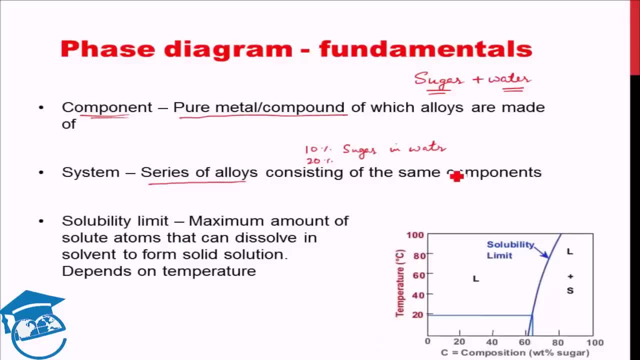 or series of solutions which has the same components. You see, the components are sugar and water, right? What we are varying is we are varying the amount of the independent components, of the individual components, And this series of different solutions represent a system of solutions or a system of alloys. 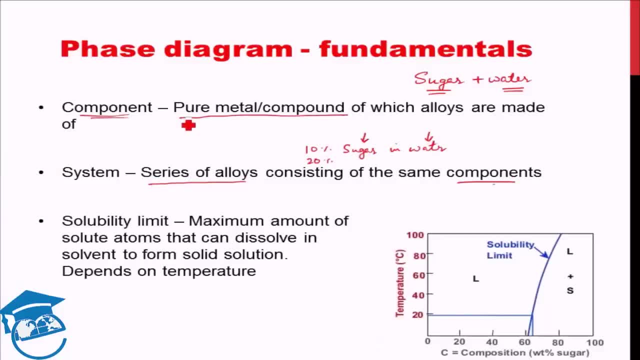 in the case of metal systems. right. So now we understood what component is. We understand what a system is. Now we need to understand something which is known as solubility limit. Solubility limit basically refers to the maximum amount of solute atoms that you can dissolve in a solvent to form a solid solution. okay, 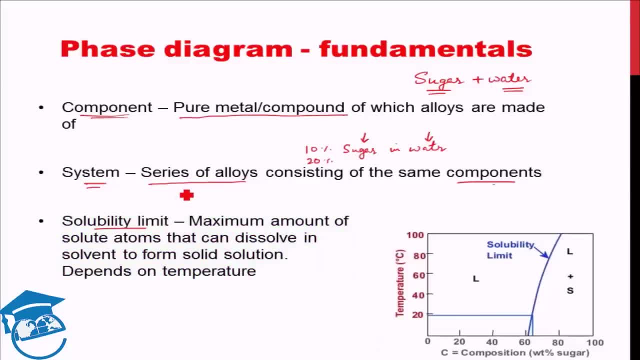 So, if you think about it, if you try to mix sugar in water, you take water at room temperature. you take one cup of water, you add one spoon of sugar, you stir it. it will mix completely. You keep on adding water. 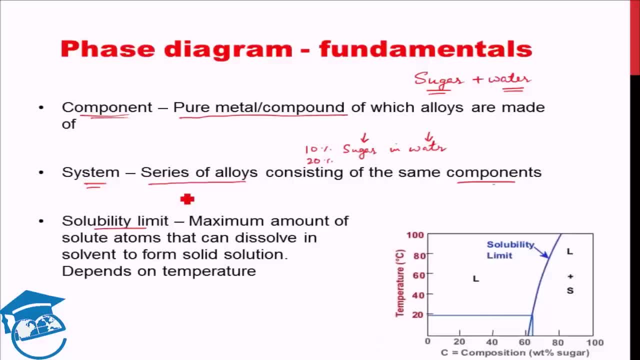 You keep on adding sugar, you keep on stirring up till one level. you can keep on dissolving all the sugar in the water, But beyond a certain level the sugar will no longer dissolve in the water. right, You will see sugar deposited at the bottom of the water which no longer dissolves in the water. 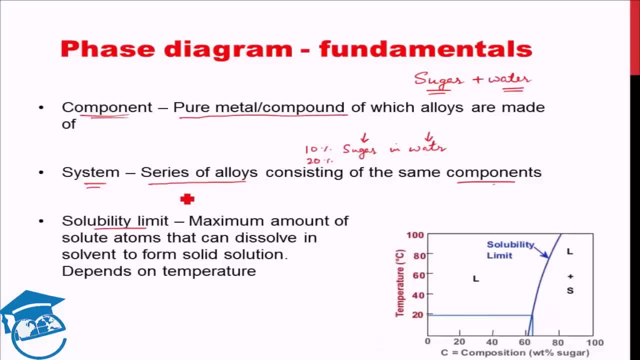 So what that means is, at that moment when the sugar stops dissolving any further, you have reached the solubility limit, which means no longer the solute that is the sugar can dissolve in the solvent that is the water. Therefore, solubility limit is a hard limit of the amount of solute that can basically 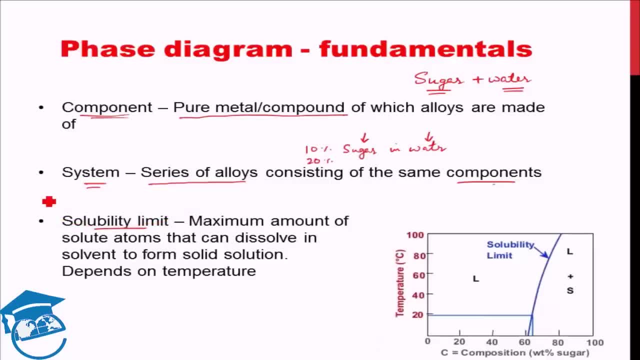 dissolve in a solvent to form a solution. But the solubility limit is also a function of temperature. It depends on the temperature of the solution Or of the solvent. How can we figure this out? In the same example of mixing sugar in water? suppose you had water at room temperature. 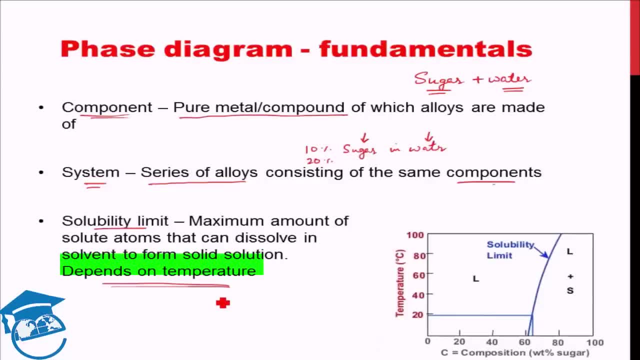 and after four spoon of sugar, the sugar no longer dissolves. Try this out. You increase the temperature, You heat the water. Then what you will observe is that now the water is able to take or dissolve from the water Further amount of sugar. 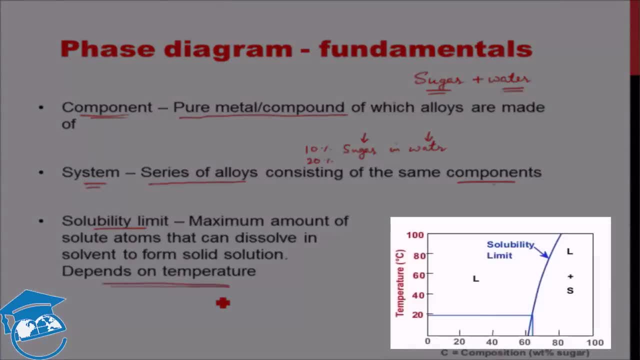 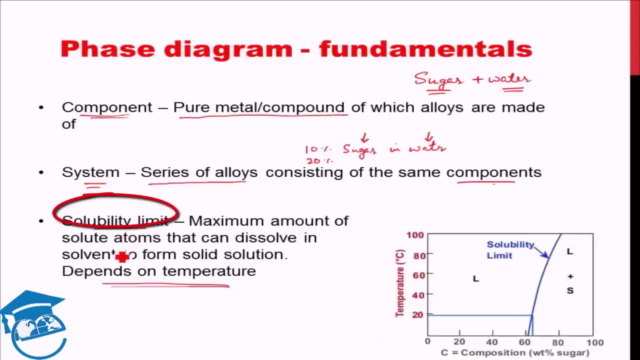 So basically, by increasing the temperature of the water you are able to increase the solubility limit, That is now more amount of solute atoms can dissolve in the solvent. That is what I mean when I say that solubility limit depends on temperature. 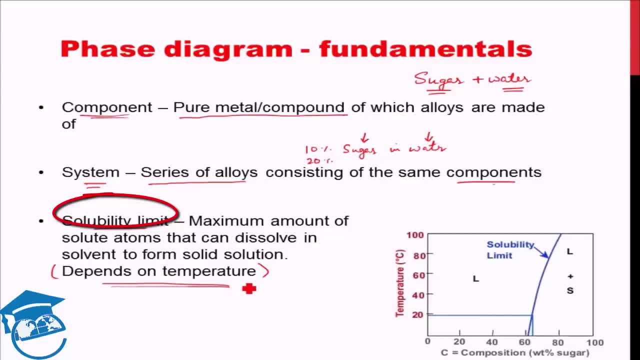 In the case of solids dissolving in liquid or solids dissolving in solid, the relation is linear. that is not linear, rather increasing. That is, with increase in temperature, the amount of solute that can dissolve increases. In the case of gases, it is normally the opposite. 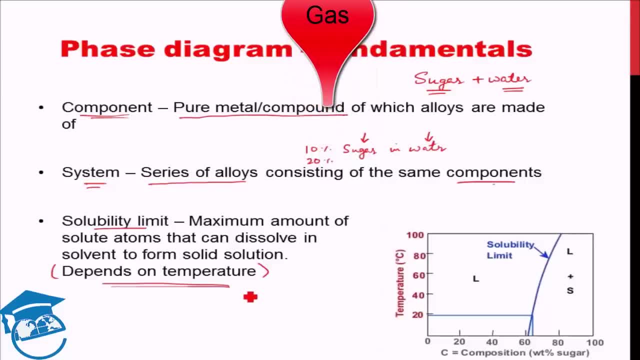 If you increase the temperature of the solution or of the solvent, then less amount of gas will be able to be retained. That is, the gas will start to evolve out on increasing the temperature. But since we will be fundamentally concerned with metals and metals, we are not going to. 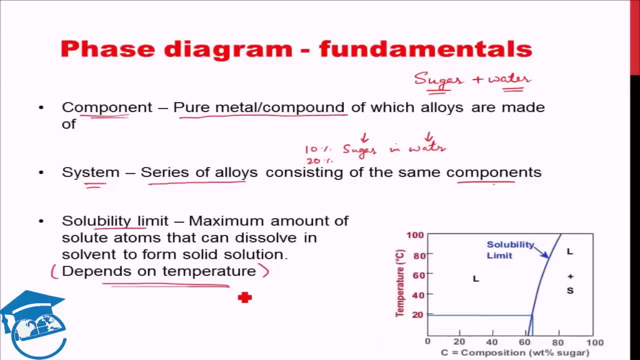 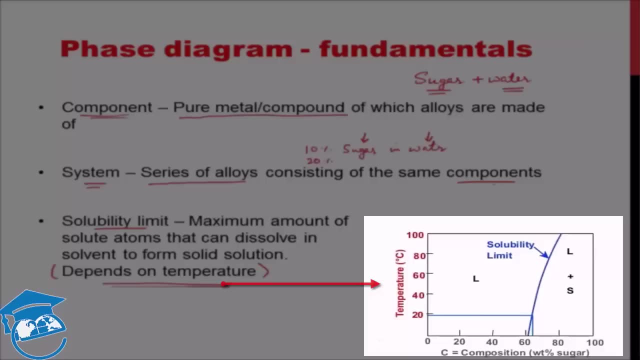 talk about metal and metallic systems, that is, solid systems. The solubility limit will be increasing in most of the cases with increase in temperature. Now let us see this diagram. This is a diagram in which we have composition, that is, weight, percent of sugar in this axis. 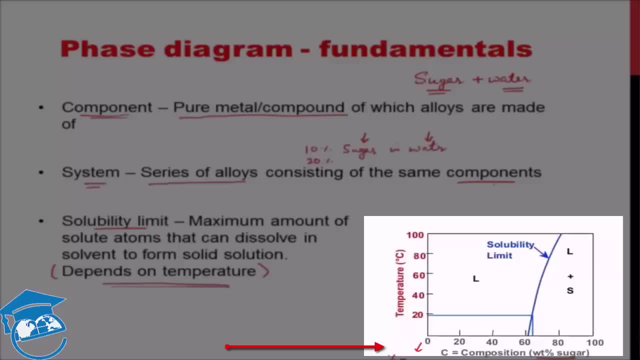 This is the composition. Over here we have 100% water- okay, 100% water- and over here we have 100% sugar. So any intermediate position: here we have 50% water and 50% sugar. This axis is the y-axis is the temperature axis. 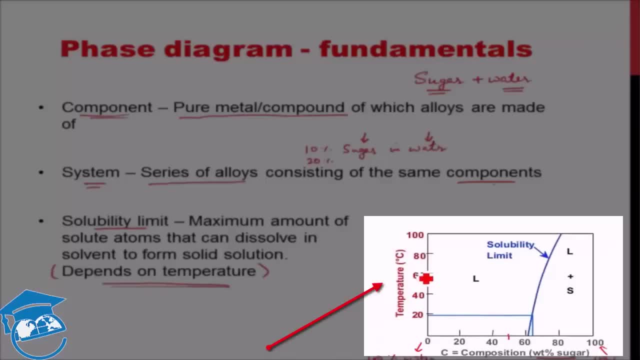 As you go up, you are increasing the temperature. What we observe is that over here, we have something written as L. This L is referred. L is referred to as the liquid. This is basically a water plus sugar solution. okay, There is no independent individual sugar left over in this region. 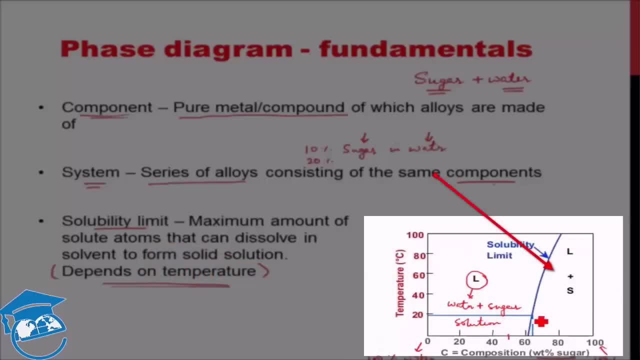 But in this region, across this line, across this blue line, here we have liquid form of water plus sugar As well as solid sugar deposited, So we have liquid plus solid. okay, And let's take any temperature. Let's say we are at 20 degree Celsius. 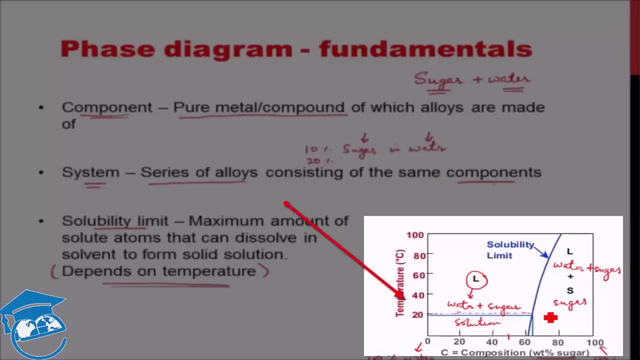 What we see from this graph is that at 20 degree Celsius we can dissolve approximately a maximum of somewhere close to 70% sugar in water. If you add more sugar, then it will deposit as sugar Solid sugar. On increasing the temperature- let's say we are at 80 degree Celsius- 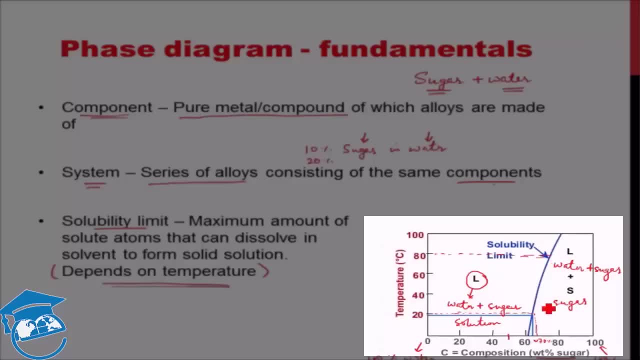 At 80 degree Celsius instead of the previous amount of 70%. now we can dissolve around 80% of sugar in water right. So this line basically separates the region. This solubility limit basically separates the region in which sugar completely dissolves. 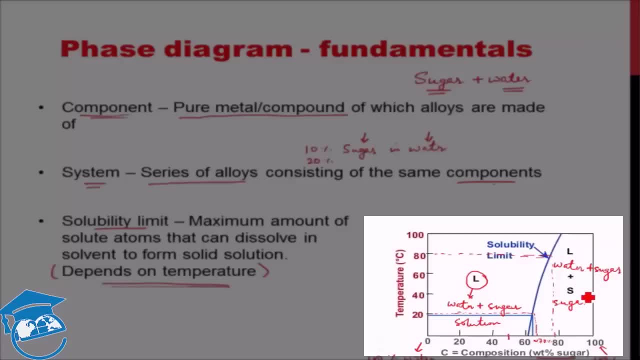 in water and the region where sugar is left over and is not able to completely dissolve in water, And this line basically represents the solubility limit line, As we'll see in further lectures. this type of representation, this diagrammatic representation, in which we have one axis devoted to composition of the components, 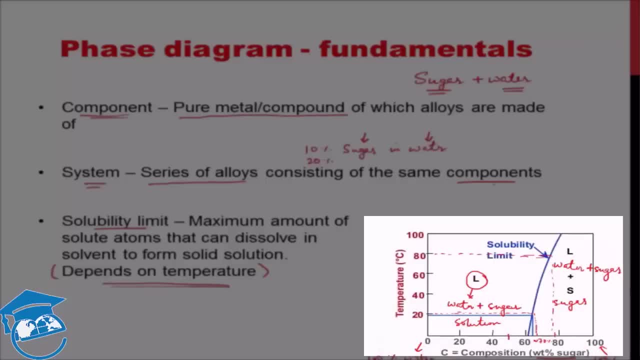 These are the components right, Water and sugar. One axis is devoted to percentage of different components And the other axis, over here, is devoted to the temperature, and over here the whole area is divided into regions having different what we'll call them as phases. 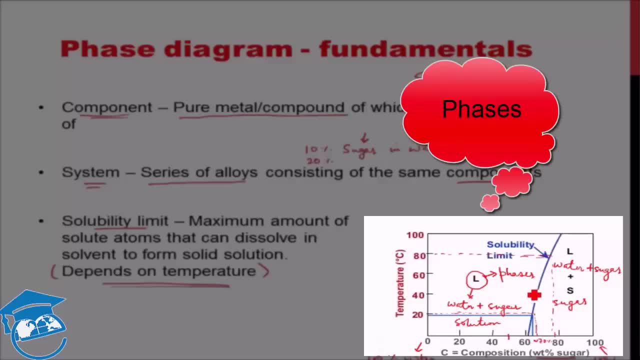 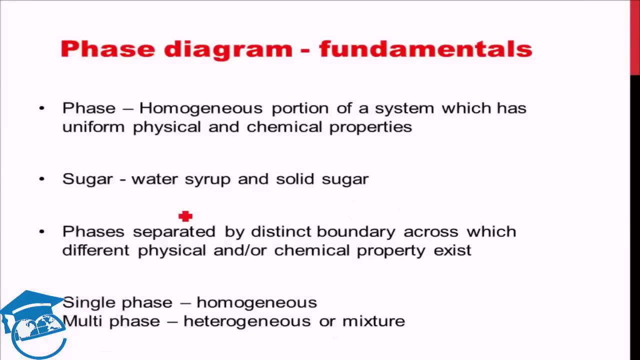 We'll see that these are phases. This type of diagram is known as phase diagram. We'll see this in much more detail. Okay, so here it is. What is a phase? A phase is basically a homogeneous portion of a system which has uniform physical and. 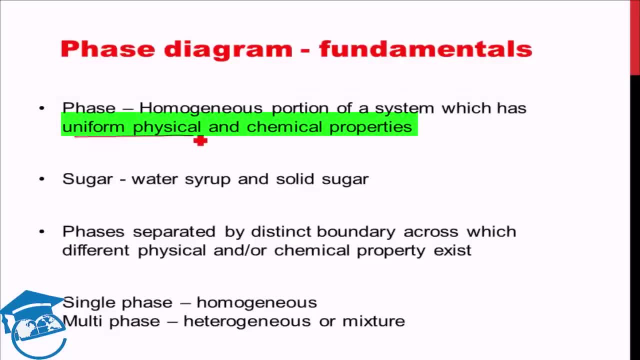 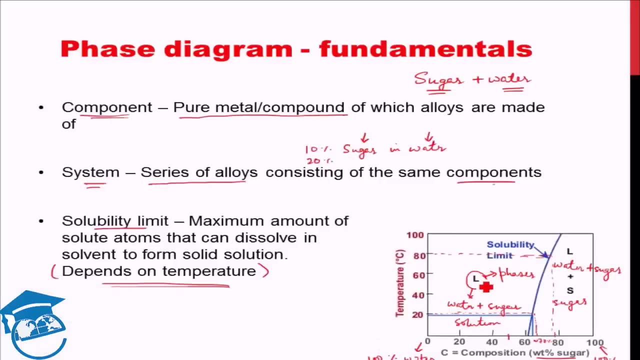 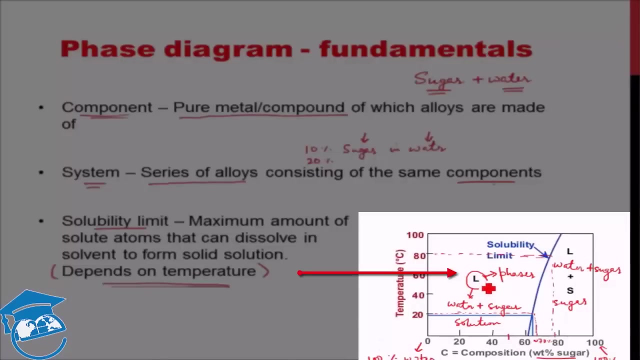 chemical properties. Uniform physical and chemical properties, That is the most important criteria for a given phase. So here what we saw is In the sugar water solution case. here this liquid or this solution basically, which had sugar and water completely dissolved, had the same physical and chemical property throughout. 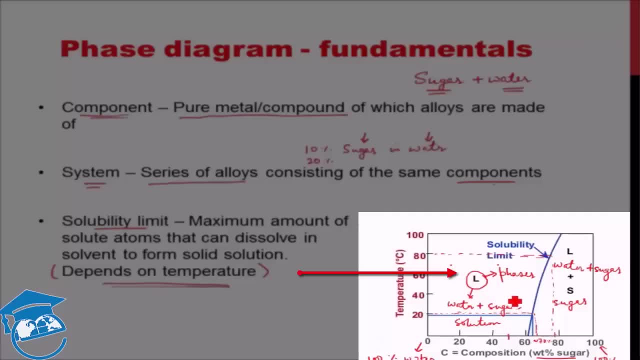 Whether we took it over here here anywhere. So this was a phase Right, Whereas in this region we had two phases. One was water and sugar solution and the other was solid sugar Which was deposited because it could not further be dissolved. 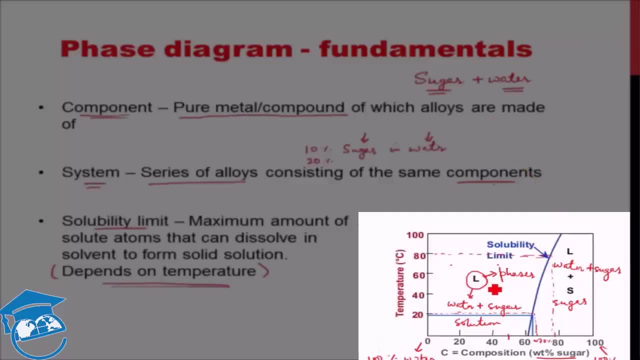 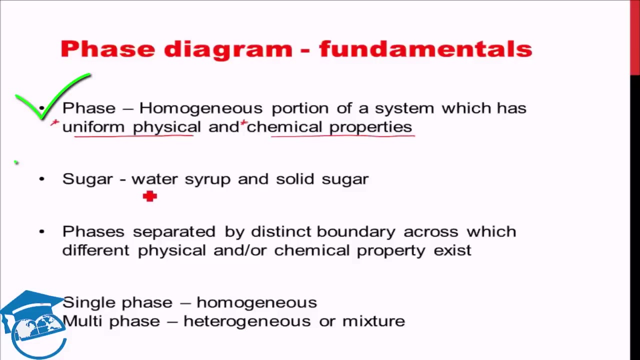 Right, So we had two phases here. We had single phase here, Whereas for both the cases we had two components: Water and sugar. Okay, Now that we have an idea what a phase is- And this is what I already discussed- that in the sugar water syrup case, if a complete 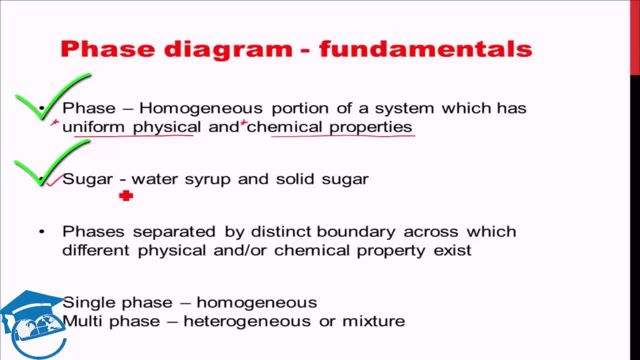 sugar is dissolved, then we have single phase. If complete sugar is not dissolved, then we have two phases. One is the sugar water syrup and the other is the solid sugar. Fine, Now how do you distinguish phases? We already know the basic definition of phase. 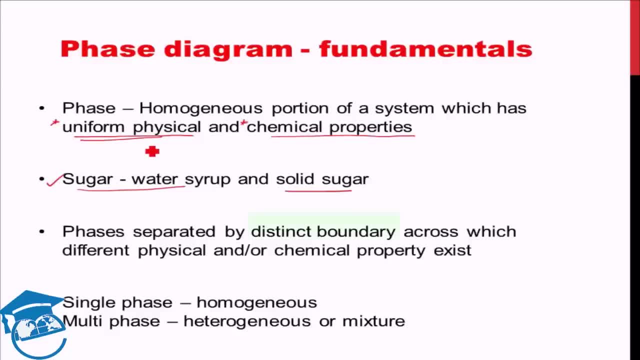 But a phase. the phases are basically separated by distinct boundaries. Right Two phases will be separated by distinct boundary. And what is the property across the boundary? Across the boundary, you will have either different physical property or different chemical property, or both of them different. 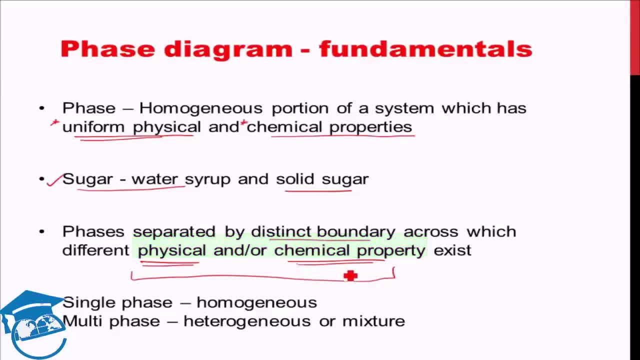 Both physical and chemical properties different. So two phases need to have at least some physical property different or some chemical property different, or both physical and chemical properties different. You cannot have two different phases, Two different phases having identical physical and chemical properties. Okay. 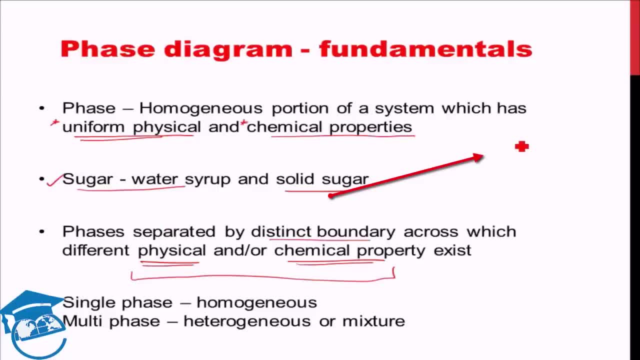 Just to give you an example: In the case of water, you can have ice, you can have liquid water and you can have vapor. Right, But these three are different phases, Though they are same component. they have the same chemical formula. 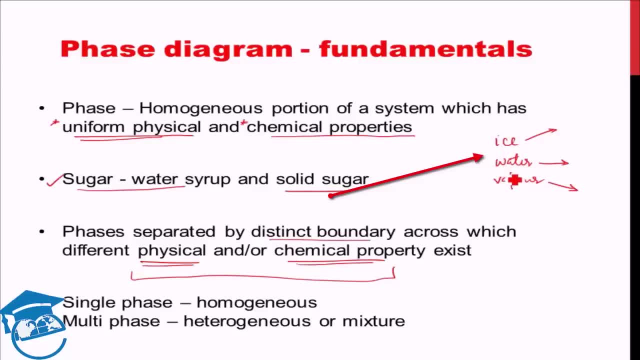 These are different phases. They will have same chemical property, that is all will be H2O, but they will have different physical properties. physical manifestation: Right, This will be in solid phase. This will be in the liquid phase. This will be gaseous. 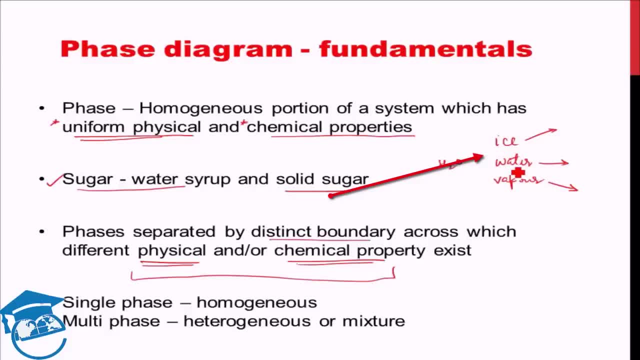 So they have different physical manifestations. Fine. Now, finally, in case there is a single phase present, In case you have a system Where there is a single phase present, Then we call it homogeneous system. Right, In case there are multi-phases present, 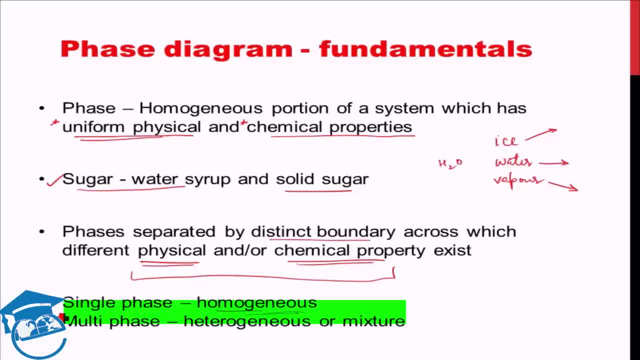 Since there is more than one phase, it is no longer homogeneous. What we call it now is either heterogeneous or it is termed as a mixture. So depending on the number of phases present, whether it is singular or plural, it will be termed as homogeneous. 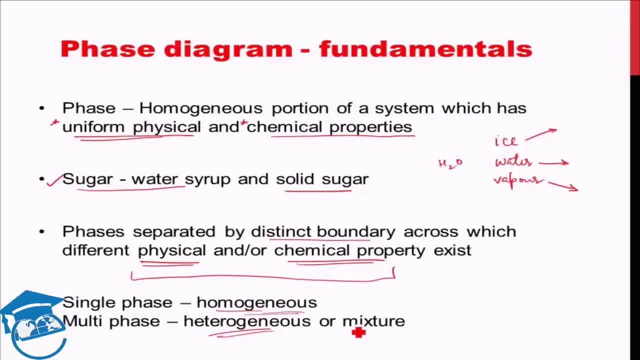 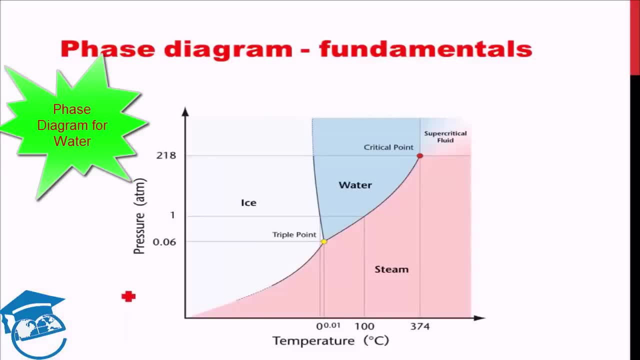 So, depending on the number of phases present, whether it is singular or plural, it will be termed as homogeneous Or heterogeneous. Okay, Now let us discuss. see the phase diagram for water. As I already said that water has, water is a single component. 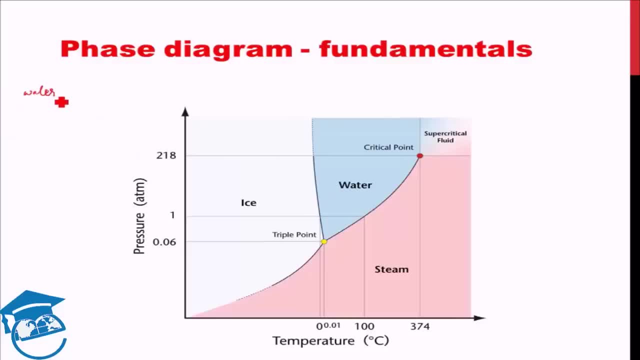 Right. Water is single component, H2O, But it has ice water and steam. Three phases present. Now what phase will be present at a particular temperature and particular pressure will be defined by the combination of the temperature and pressure. Okay, Here in this phase diagram, we have one axis for temperature, the other axis for pressure. 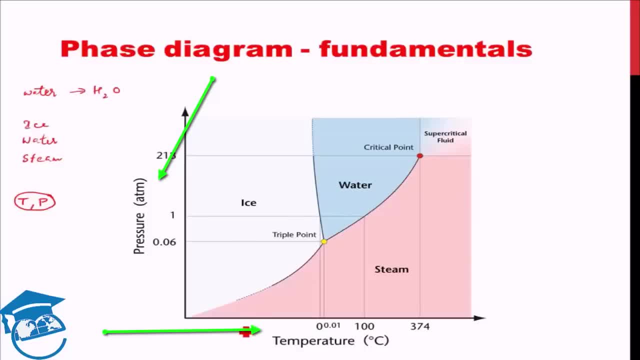 There is no axis for component percentage because it is single component, It is always water, 100% water, So we do not need a Component percentage. axis will have a temperature axis, a pressure axis And, depending on the combination of temperature and pressure, we'll get whether we'll have 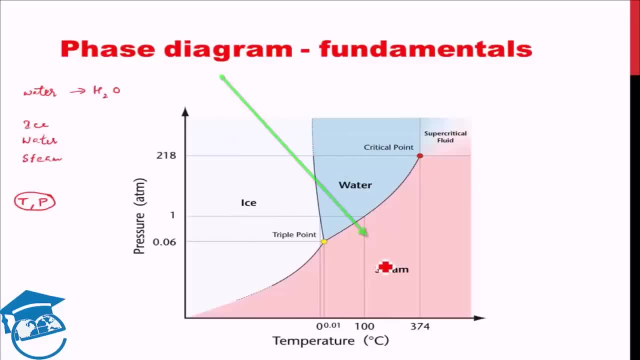 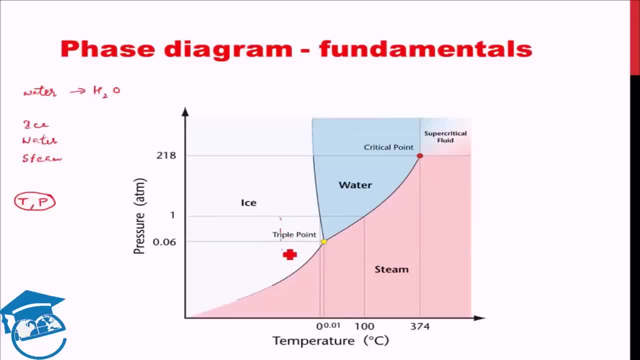 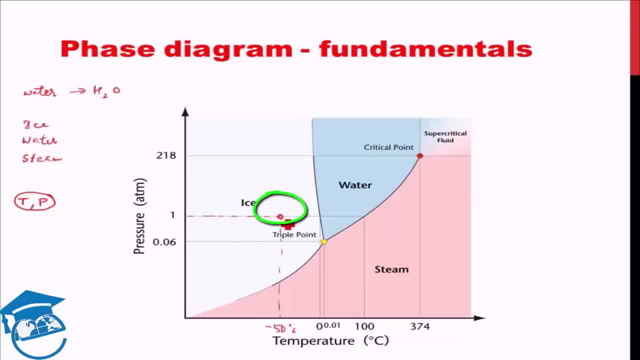 We end up in this region, right, And this region, as we can see, is the region for ice. By our experience, we know that at minus 50 degrees Celsius we are supposed to have ice and nothing else, given that the pressure is atmospheric pressure. 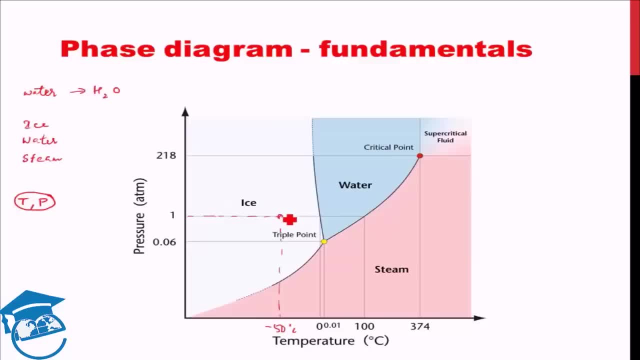 Now suppose that you take this. you keep the temperature at minus 50 degrees Celsius itself, But you start reducing the pressure. You reduce the pressure so low that you enter this pink zone. Suppose you are over here at this pressure. Then what will happen? 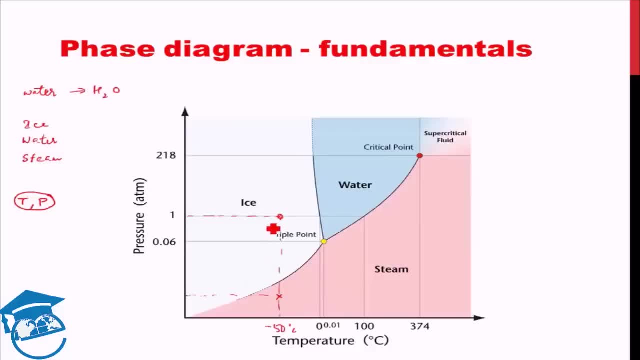 What is basically happening is that the ice is getting transferred or converted into steam. Okay, Why so? Basically, vapor exists when the vapor pressure is able to overcome the atmospheric pressure Right, And any solid has some vapor pressure associated with it. So ice also has some vapor pressure associated with it. 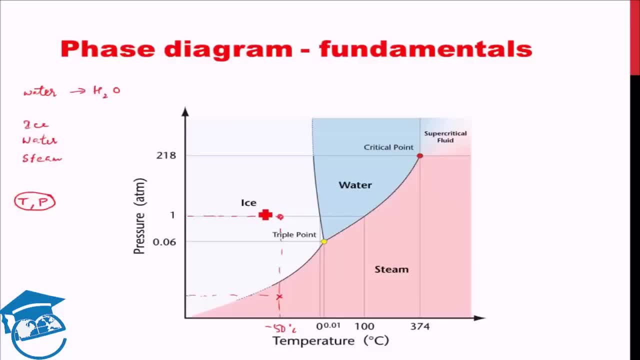 Because there are atoms on the surface which are, which may come off and provide some amount of pressure right. Similarly, liquid water has also some vapor pressure associated with it. Therefore, what is happening over here? that the atmosphere pressure is coming so low that 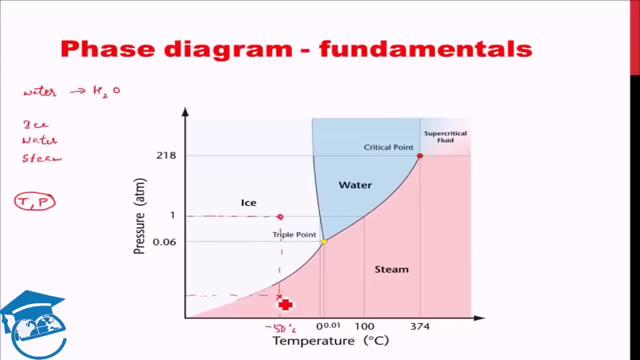 the vapor pressure of the atoms from the ice is exceeding the atmospheric pressure, Thereby the solid ice is converting into vapor steam. So here you can see the different phenomena actually happening, How you can tweak the pressure and temperature combinations to get a different phase altogether. 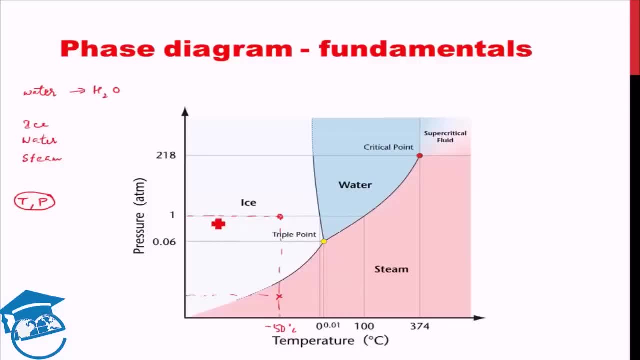 Okay, Now let's jump into the water region. If you keep one atmospheric pressure, but you go to zero degree Celsius, We know that at zero degree Celsius we have water as well as ice present, Right? So if water as well as ice is present at zero degree Celsius, that is exactly what. 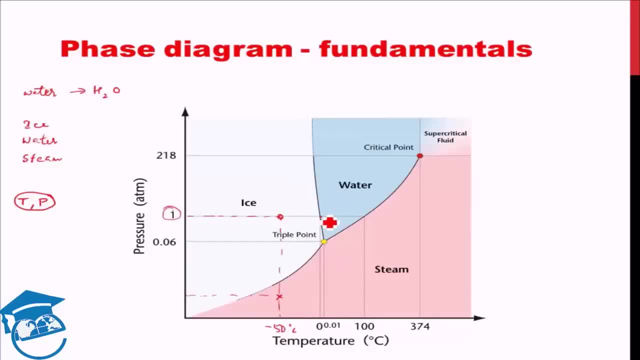 is happening here: Zero degree and one atmospheric pressure is falling at the interface of water, ice. Therefore, over here we will have both water and ice. Increase the temperature further. you reach a hundred percent water. Take that temperature to a hundred degrees Celsius. 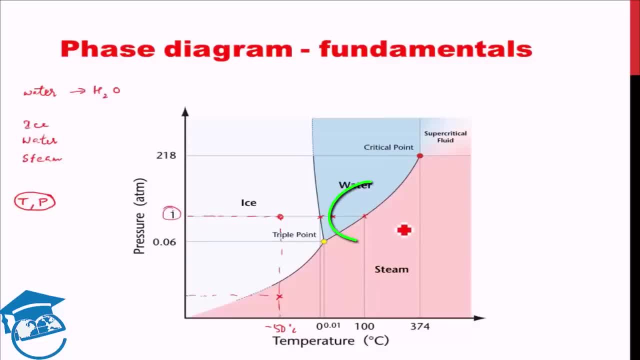 Now you are at the equilibrium of water and steam, So you will have, at a hundred degrees Celsius and one atmospheric pressure. both water and steam increase the temperature further and we get complete steam or complete water vapour, Right. So this is how increase of temperature affects the phase changes and that can be deduced. 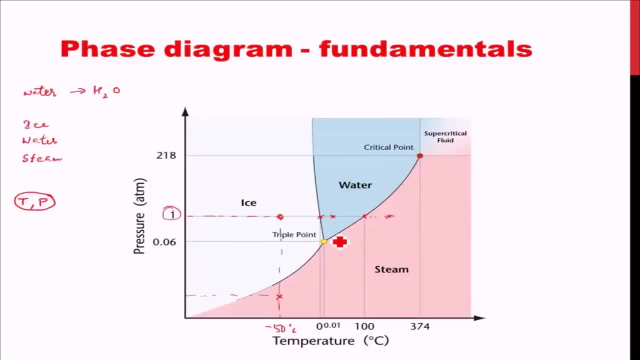 from this phase diagram. I would like to draw your attention to a few important details here. One is what is known as triple point. Triple point or it's also called invariant point. You will encounter invariant point several times when discussing phase diagrams further, But for water it is called triple point. Triple point is the combination of: 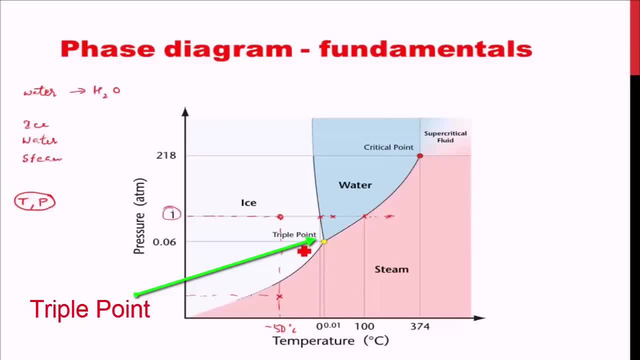 temperature and pressure at which all the three phases co-exist. So, at 0.06 atmospheric temperature and 0.01 degree Celsius temperature, we have ice, water and steam, all of them three co-existing. That is seen here, because all the three lines meet at this point. Okay, Then we have this: 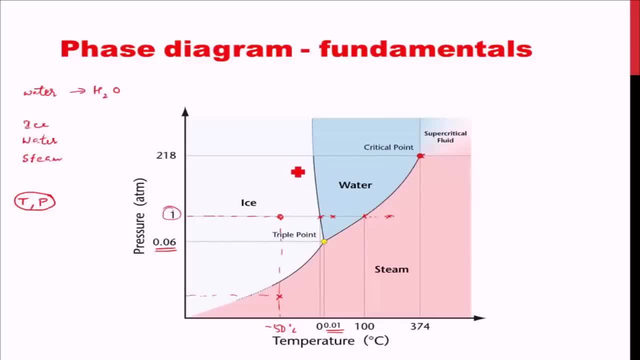 point, that is, 218 atmospheric pressure, very, very high pressure and 374 degree Celsius, quite high temperature Over here. beyond that, you will have something which is known as supercritical fluid. Supercritical fluid is basically something which has properties of both a liquid and vapor phase. We will not go into details of that. You can study up. 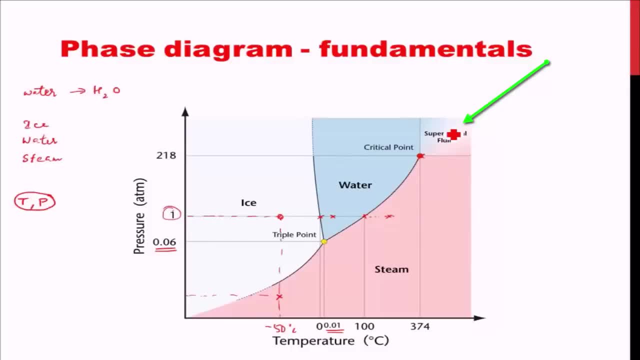 more about supercritical fluid if you want, But we do not need for our understanding any further. The only take home is: supercritical fluid has properties of both liquid and vapor state co-existing, And that temperature and pressure combination is known as critical point, beyond which we have supercritical fluid. 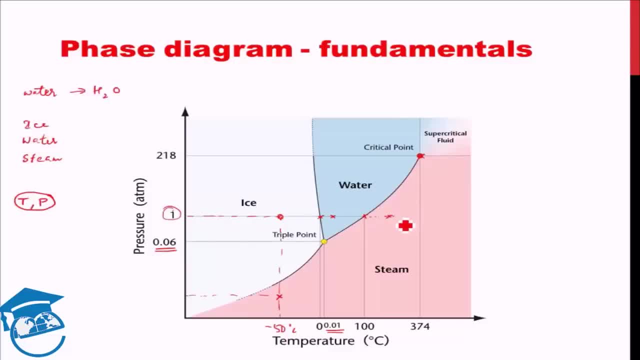 Okay, So this gives you an idea about phase diagram fundamentals. Here again, what we see is that we have distributed the temperature pressure area into different regimes, having different phases existing, And we have boundaries along which phases co-exist Right With this background, 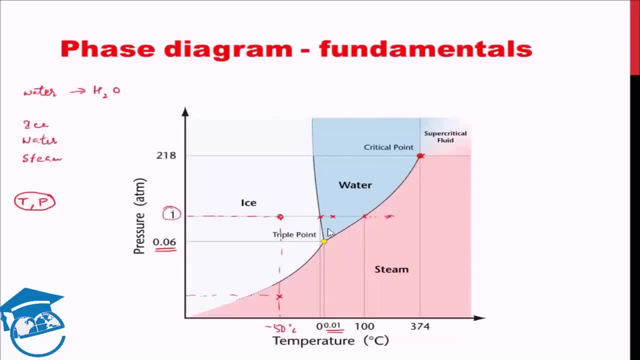 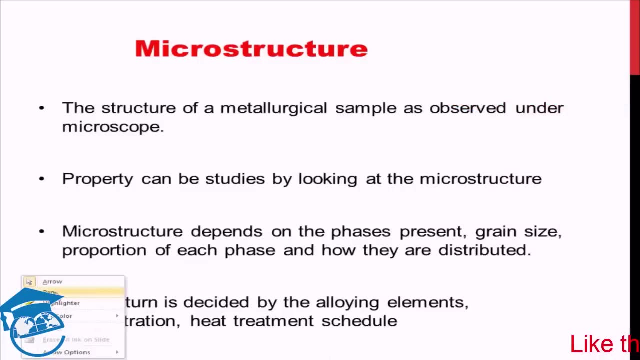 let us understand what is microstructure. So let us give you a brief understanding about phase diagram. Now let us see microstructure. Microstructure is one of the most important things that you need to understand while understanding metallurgy and material science. Microstructure is basically, as the name suggests, micro. that 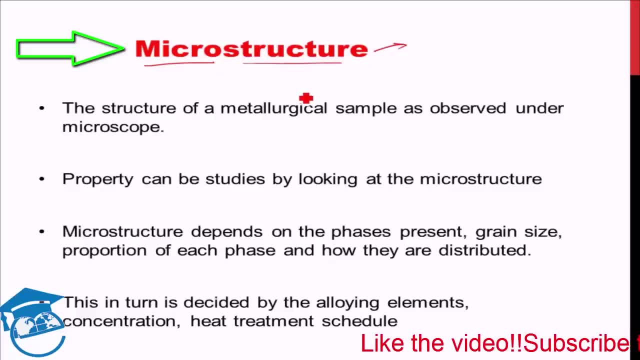 is small structure. It is the structure as observed under a microscope. What is the importance of a microstructure? Microstructure: by studying it, we can predict what is the property of the material at hand. The property is influenced drastically by the nature of the microstructure that exist. 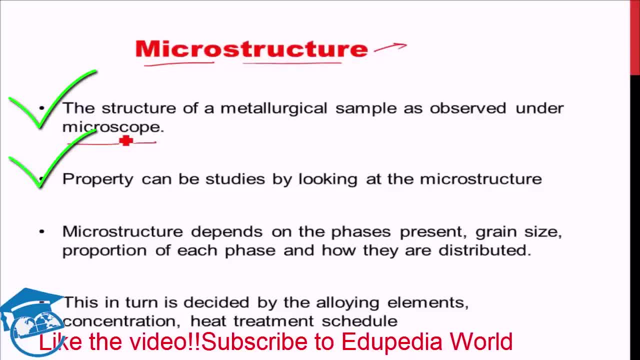 Okay, Now what are the different components of a microstructure? When you see, let us say, a steel sample under a microscope, you will be able to see the phases, different phases present, able to identify what is the grain size of the different phases present. They will be: 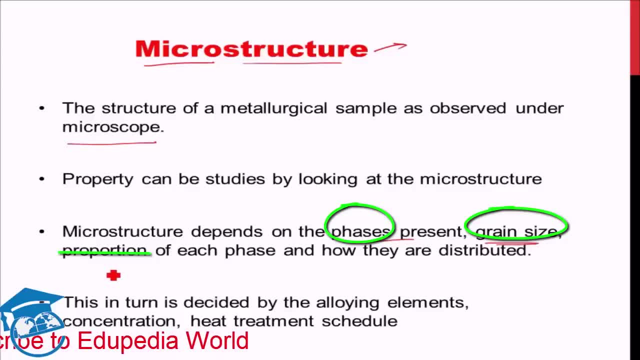 also able to observe. what are the proportion of the different phases present, How much is each phase present And how are they distributed? How are the different phases distributed? What is the shape of the different phases? Is it needle like? Is it equiaxed, Is it elongated? 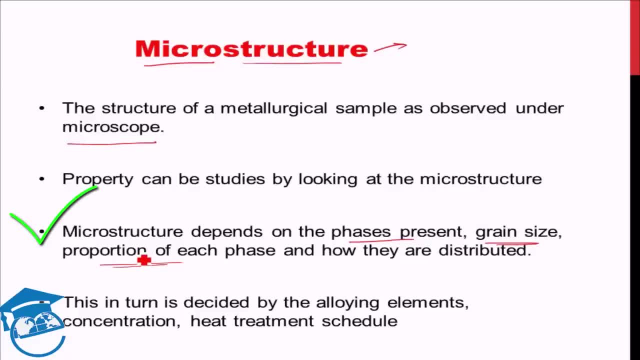 Everything together, all these properties, all these observations together lends to the ultimate property that the material will have. But what are the things that decides these parameters? What is it that decides what will be the phases present, The grain size, How much amount of different phase will be present? That is kind of dictated by several things. 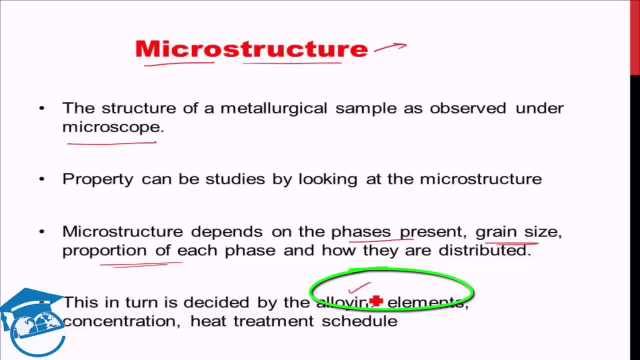 One is: what are the alloying elements present, Like if you have a steel, whether there is chromium present or not, whether there is boron present or not. what are the alloying elements present that will affect the arrangement of the phases and the phases? What is the? 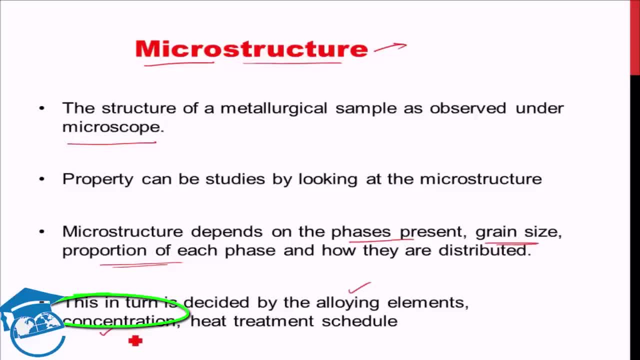 concentration of the alloys that you add. Are you adding 2% chromium? Are you adding 10% chromium to it? That will affect the microstructure. And, last but not the least, and one of the most important thing, is the heat treatment schedule that you are undergoing. You take 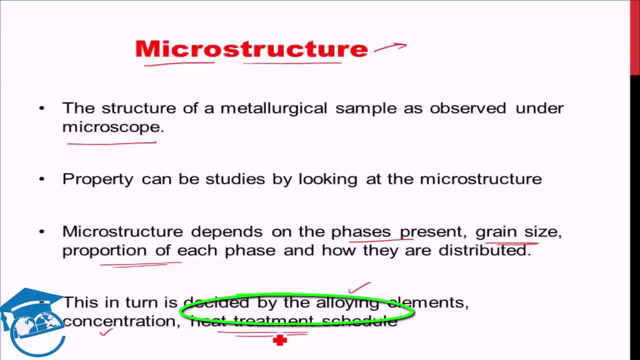 a steel, you take it to 800 degree Celsius and you cool it rapidly in ice cold water. Alternatively, you take a steel, you heat it to 800 degree Celsius and you let it furnace cool. that is, it cools very, very slowly. These two are two completely different kind of heat. 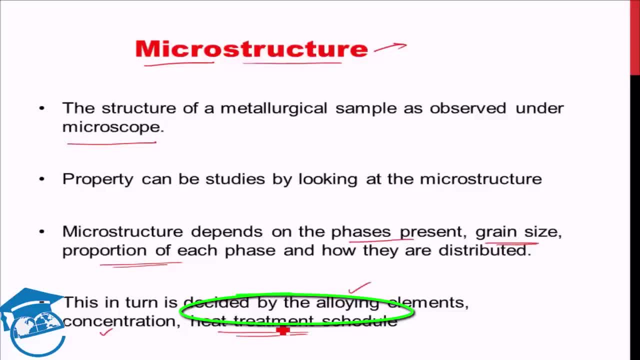 treatment schedules right, And this difference in heat treatment schedule will lead to completely different microstructure, thereby completely different properties. So the take home here is that microstructure dictates property and the microstructure itself is dictated by several factors, including the alloying element, their concentration and 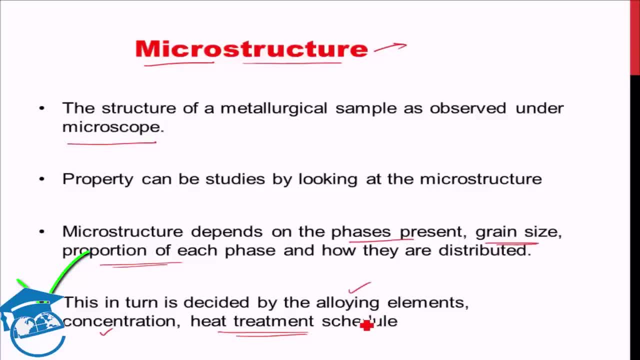 the heat treatment schedule that you follow, Among which the heat treatment schedule is one of the most important, because you are able to Form the heat treatment schedule as per your requirement. You cannot change the alloying elements as per your requirement, always Okay. Now these are two examples I have put up just 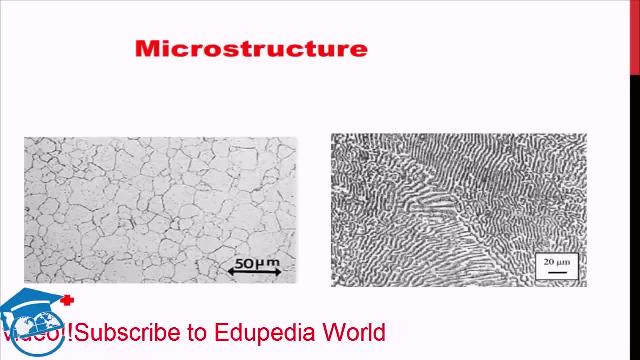 to show you how microstructures look. How are different microstructures look? Does different microstructures look? This is copper. To give you an idea, this is 50 micron. This is about the thickness of a hair, single hair. This is quite a magnified view. This is copper single phase. You can see these are different. 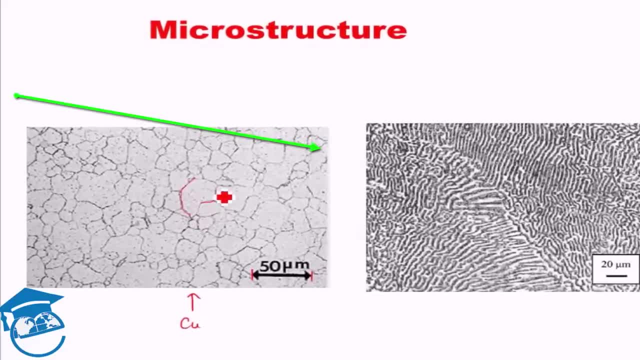 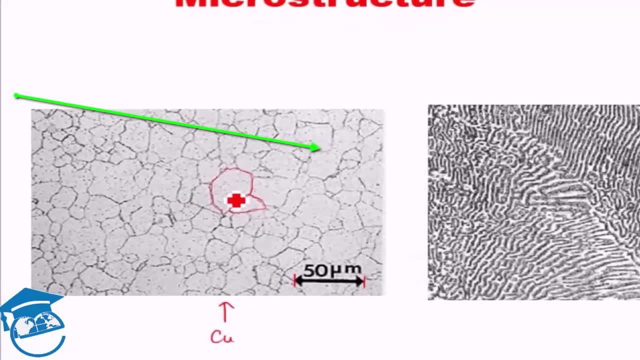 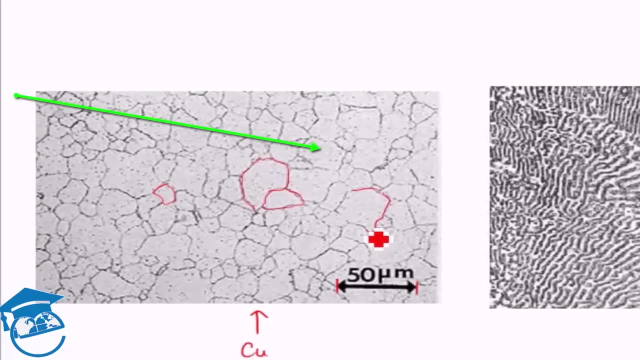 grains. This is one grain of copper. This is a different grain of copper, right? So what we see is that not all grains are equally sized. Some are quite small grains, Some are relatively large grains, But the average size will tend to be close by The median size.